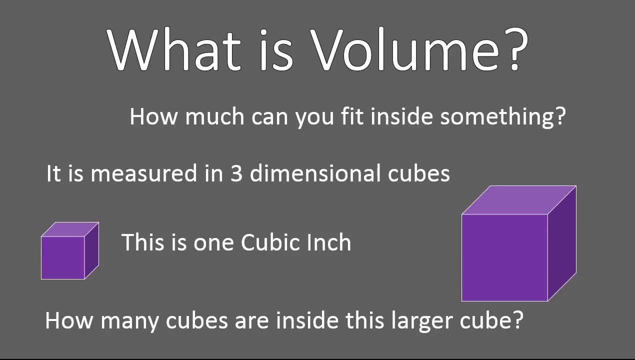 How many of the smaller cubes can fit inside this? And then I'd start kind of placing the smaller cubes inside there: One, two, three, four, five, six, seven, eight. So there's eight cubic inches inside of this larger cube And that's the basics of volume. How many cubes can fit inside of other objects? Not 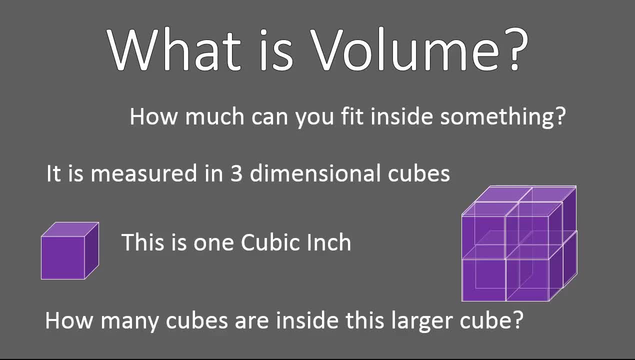 always cubes, but different objects. Any three-dimensional solid. we say how many cubic inches or cubic centimeters can fit inside of it? And then we'd start kind of placing the smaller cubes inside of that larger cube. How many cubic feet can we fit inside of that? So it's measured in three. 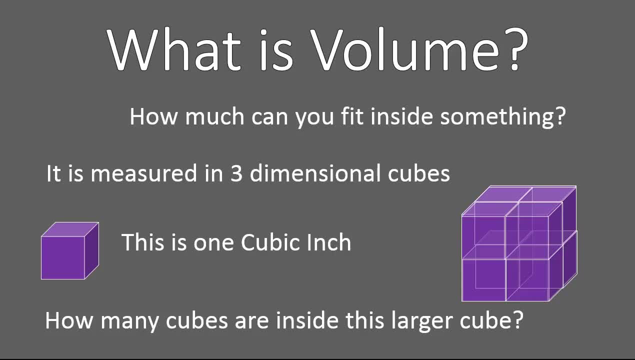 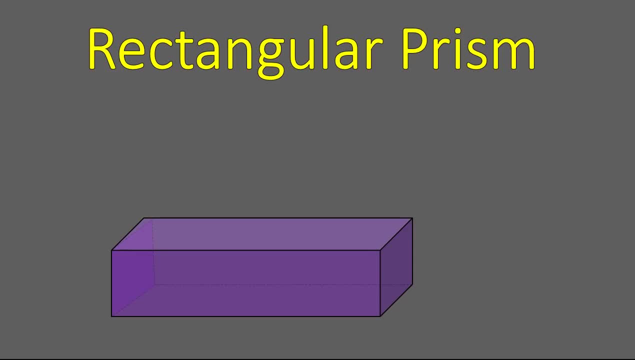 dimensions. It's measured in cubic units. whatever the unit of measurement is, And it is like that. All right, Let's talk about one shape specifically. This polyhedron is called a rectangular prism. A rectangular prism is like this: It has rectangles on the sides of the 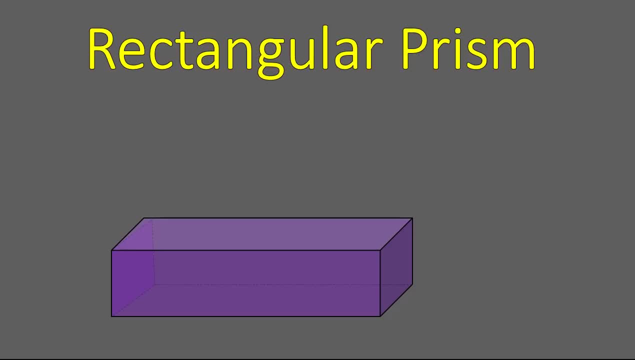 figure. At least two of the sides are rectangular that are opposite each other, which makes basically all of the sides either rectangular or it could be a square on the end, But they're going to look like this. This is a rectangular prism And all of the angle measurements are 90 degrees, That's. 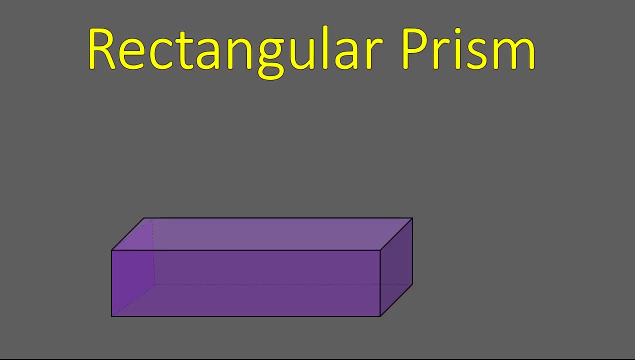 kind of a given with rectangular prisms. So with a rectangular prism, when we're trying to calculate the volume, we would use this equation: The volume is equal to the length times the width times the height, Where this is the length, this is the width, and 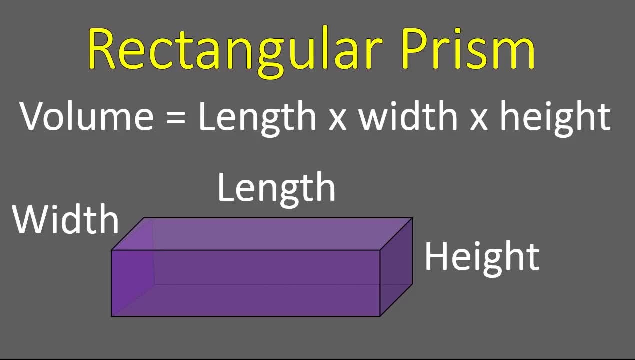 this is the height. Now, if you forget which one is length and which one is width and which one is height, it doesn't matter, because you can really turn this on end and then it would change all of them And because we're multiplying, it doesn't matter what order you do them in. 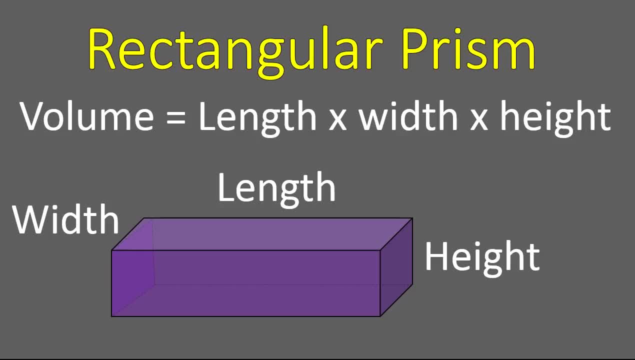 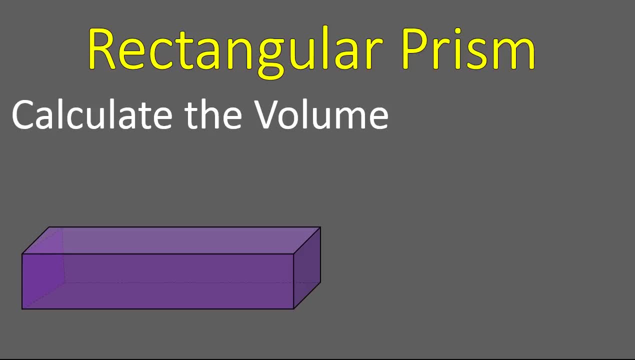 So all you have to remember is that the different measurements you're given, you're multiplying them all together. So let's do one quick here. example of a rectangular prism. So let's do one quick here: example of a rectangular prism, calculating the volume of this rectangular prism when you're given three. 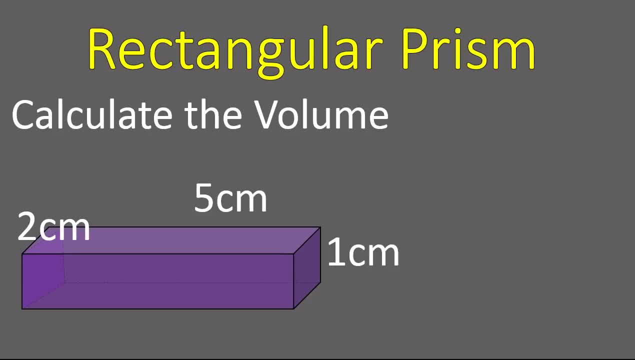 measurements. This: 5 centimeters is our length, 2 centimeters is our width, 1 centimeter is our height. So our volume is the length times the width, times the height, And I would write that out as 5 times 2 times 1 and calculate that as being 10 cubic.